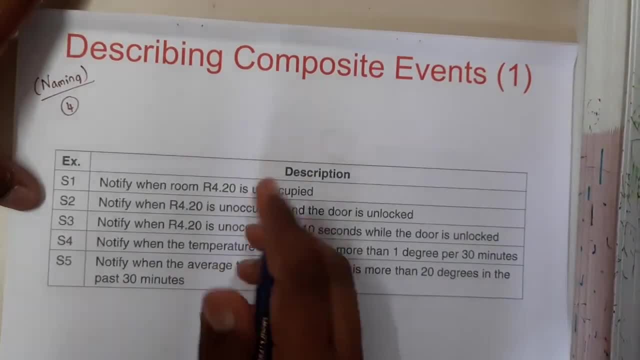 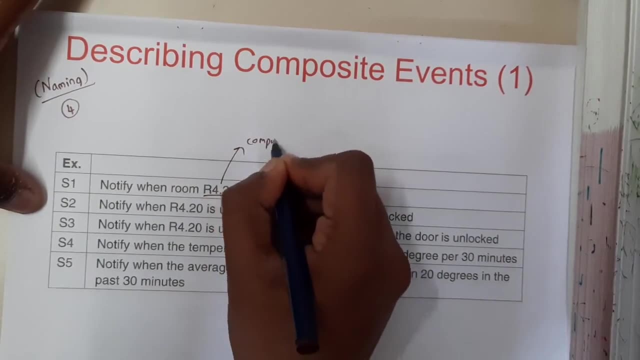 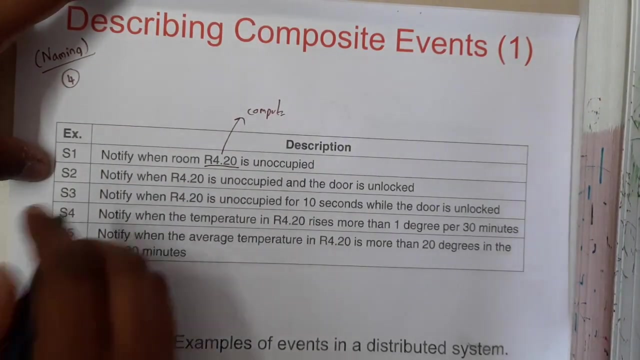 I do not want to give wrong information. So basically in this example this R44.20 is a computer guys or a computer or a system or a device. you can say So. here in this table they are representing the events with that description. So whenever event S1 occurred, 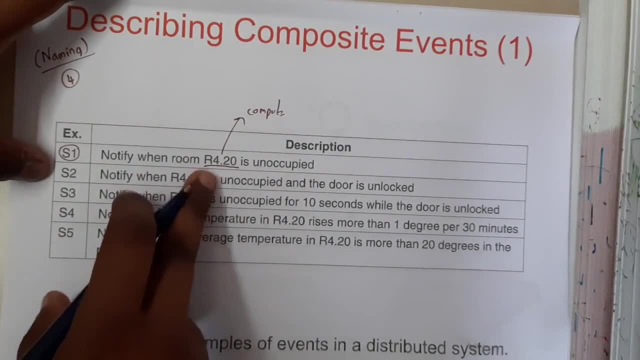 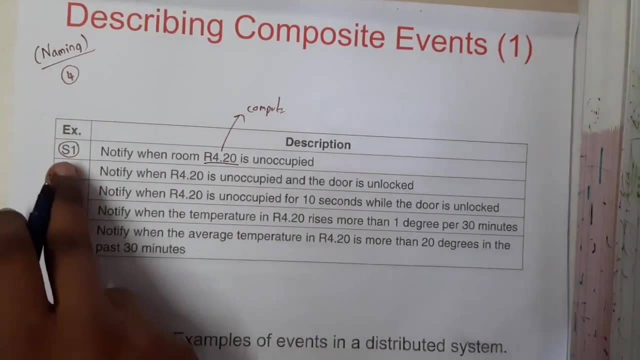 so there you are saying that, notifying when a room of R4.20 is unoccupied. So the room which you have allocated for that system is empty. That is what it is indicating with S1.. Similarly with S2, we are notifying it is unoccupied. 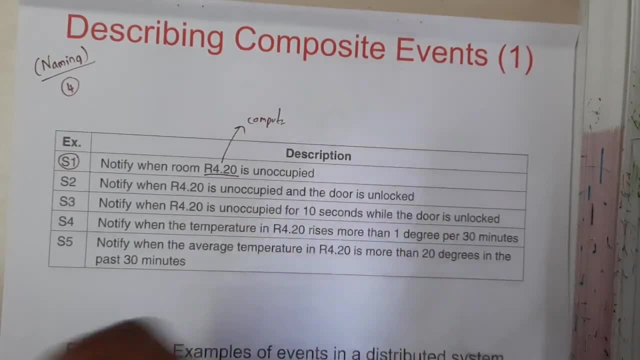 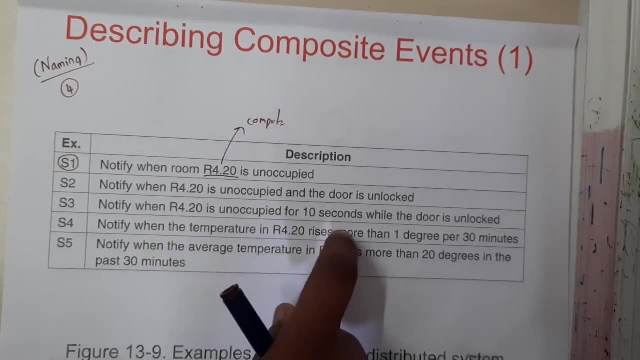 and the door is unlocked. So basically, the door is not locked. Someone can enter inside. So you are indicating it Similarly. S3, notifying when R4.20 is unoccupied for 10 seconds while the door is unlocked. So basically, it is unoccupied only for 10 seconds and the door is unlocked. 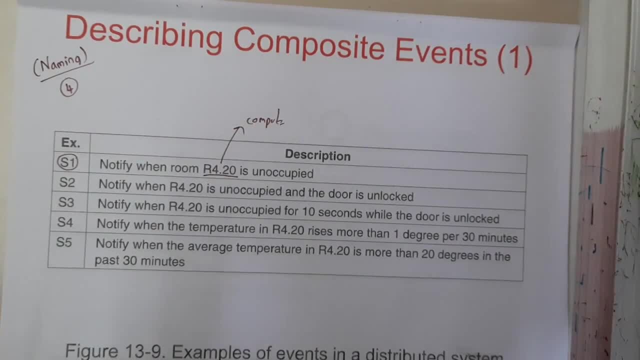 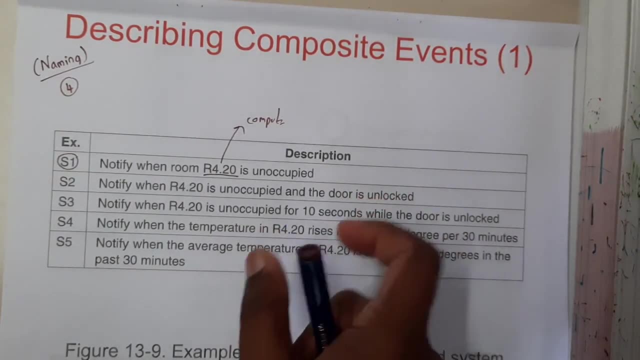 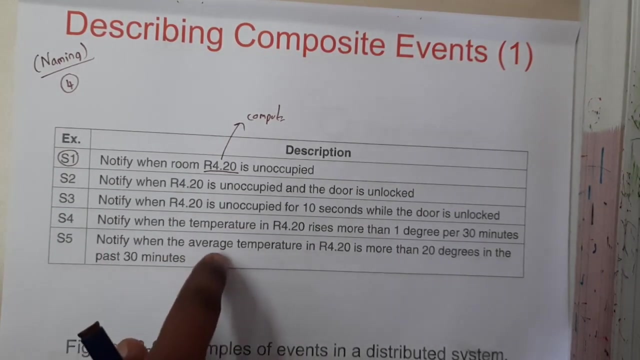 So something could have happened. Similarly, S4, notifying when the temperature of R4.20 rises more than 1 degree per second For every 30 minutes. if the temperature is increasing by 1 degree, then you will be notifying him. Similarly, S5, it is nothing but notifying the average temperature in the room. 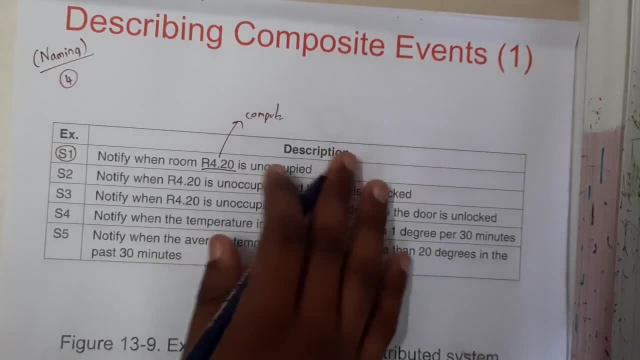 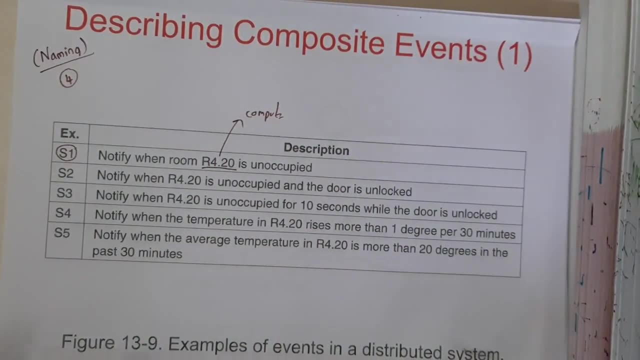 is more than 20 degrees in the last 30 minutes. So basically, in simple words, you can say: based on some particular events, you will be sending some messages. So that process is nothing but naming guys. So this is called as composite events. So if you want an example, so assume. 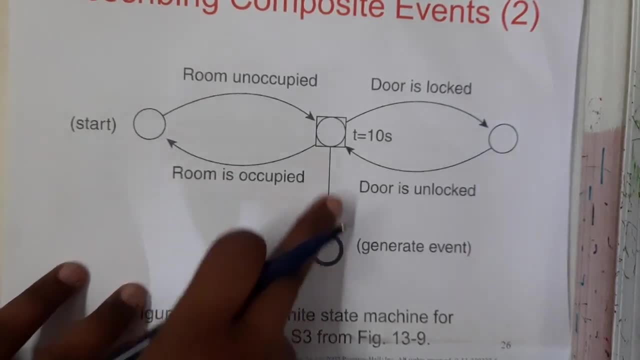 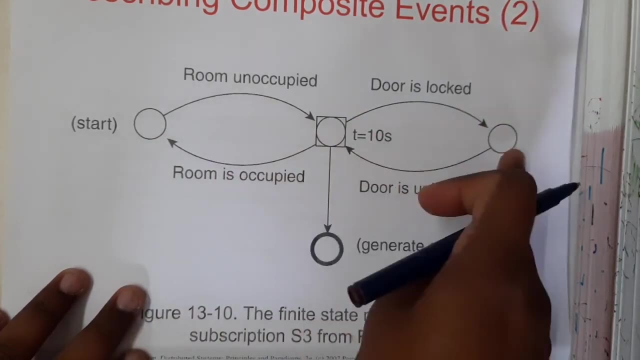 that this is your event generator guys. So this is your room and this is your staff. So basically, you will be checking. the room is unoccupied, Then you will be locking it, Then you will be unlocking it, Then you will be occupying it So you can do any kind of operation with the room, So you can unlock. 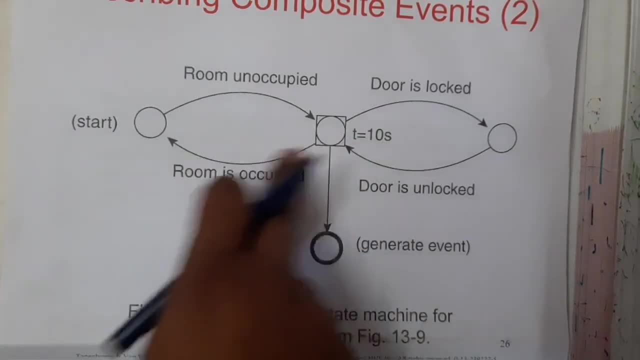 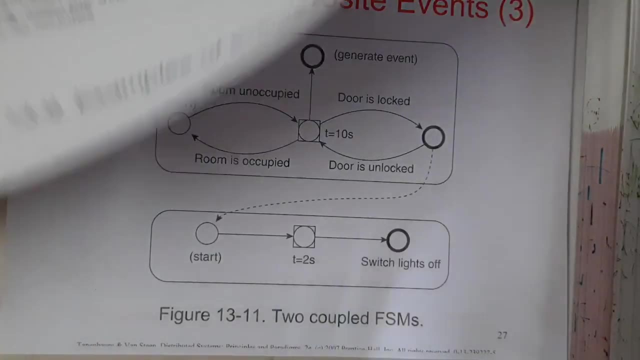 it, occupy it, unoccupy it, lock it, unlock it. So, based on your operations, the events will be generated. So this is the finite state machine for subscription of S3.. So, basically, here we draw on for S3. for this, For 10 seconds, it should not be on, because, if you notice,